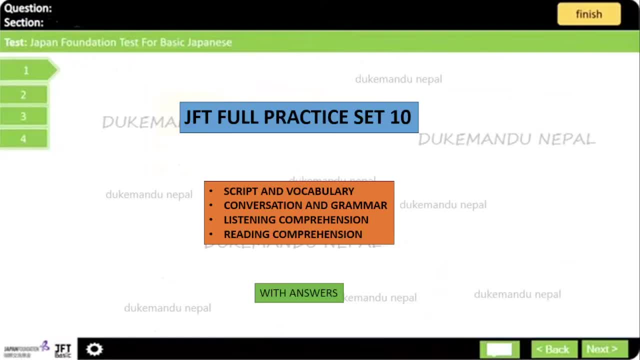 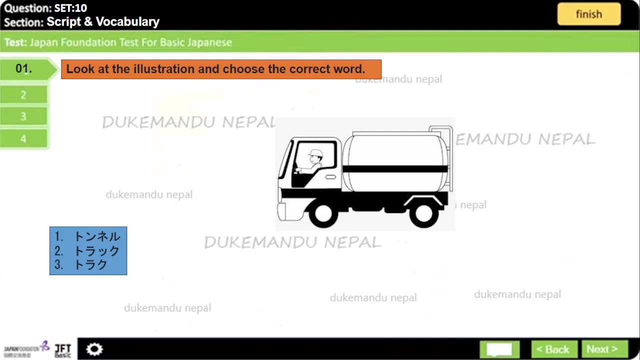 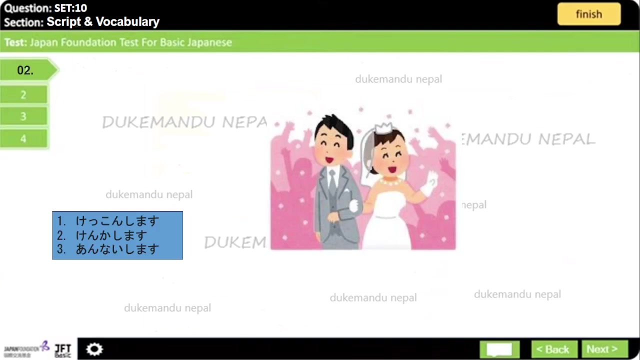 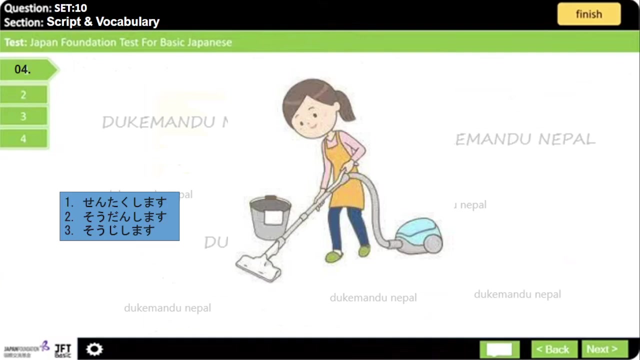 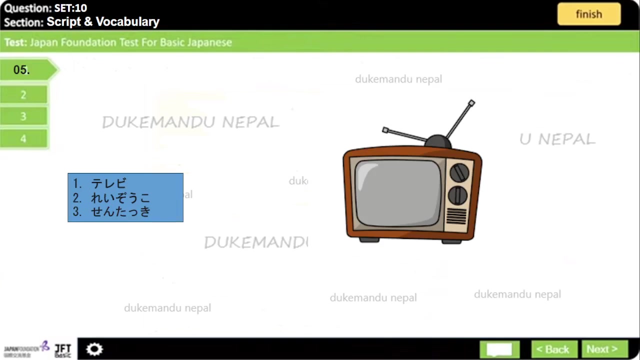 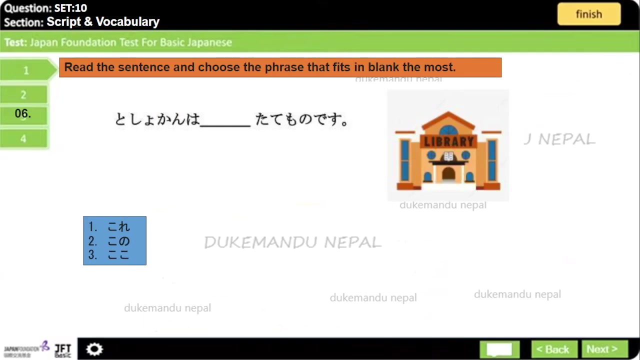 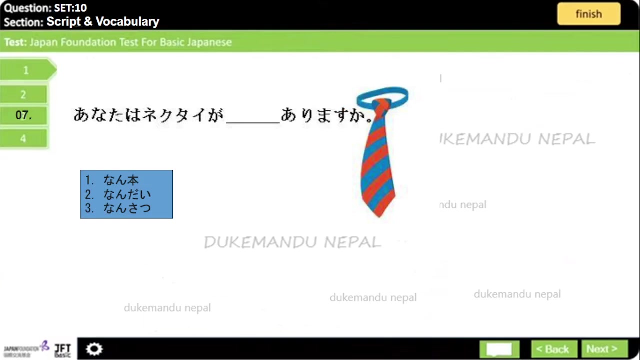 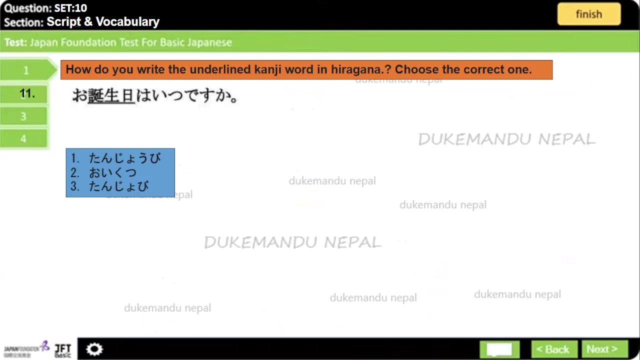 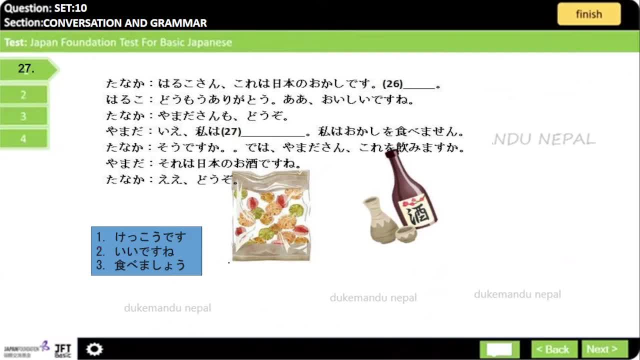 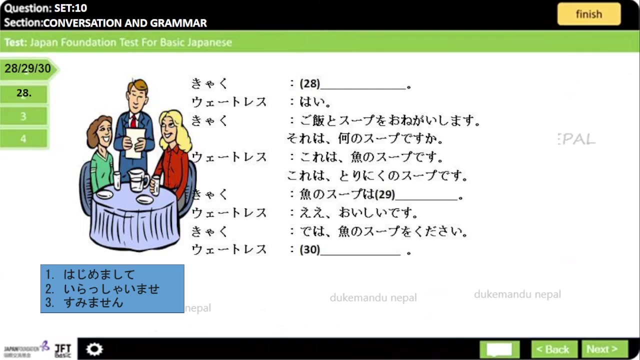 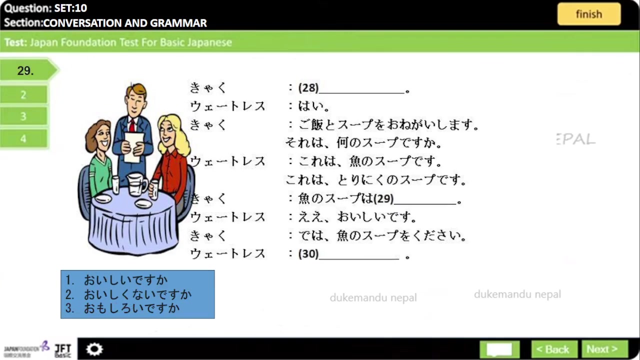 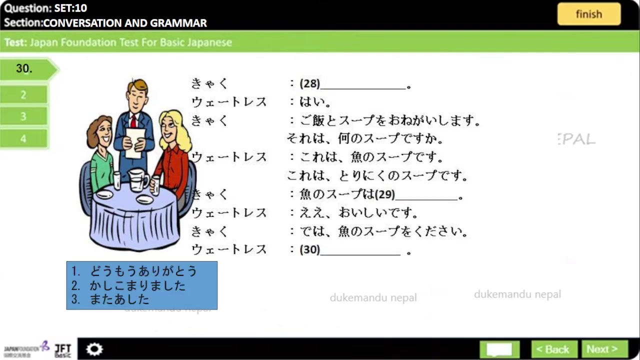 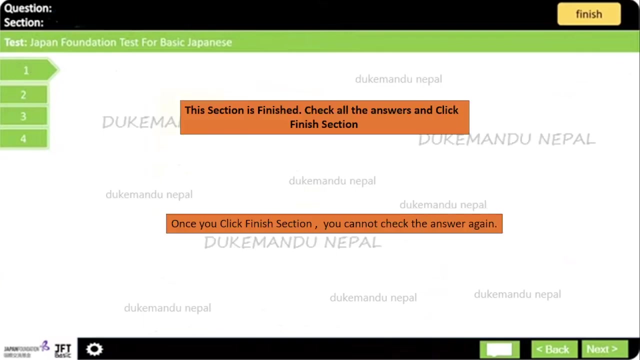 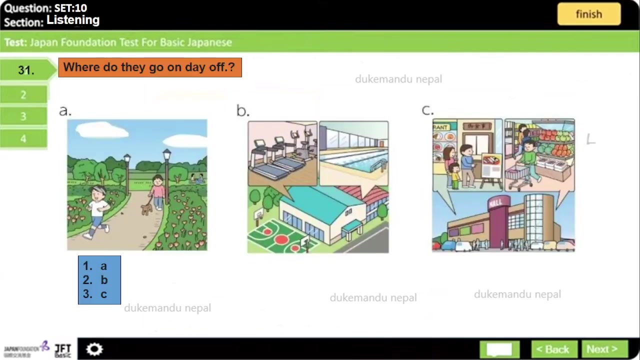 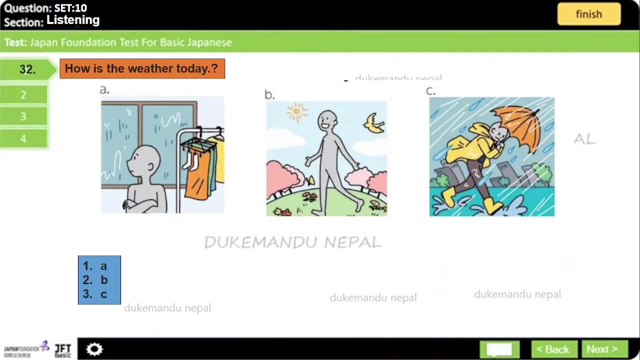 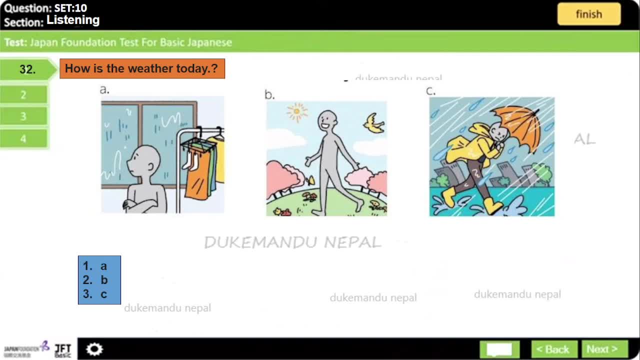 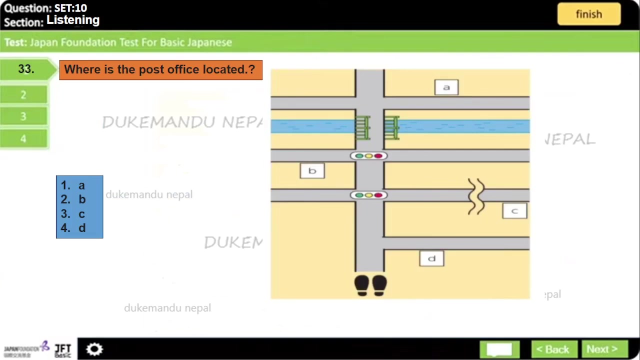 Good morning. It's a nice day today. Yes, it is a nice day, It's gotten a lot warmer. Yes, it is Sorry to keep you waiting. It's not your birthday, It's my birthday. Sorry to keep you waiting. 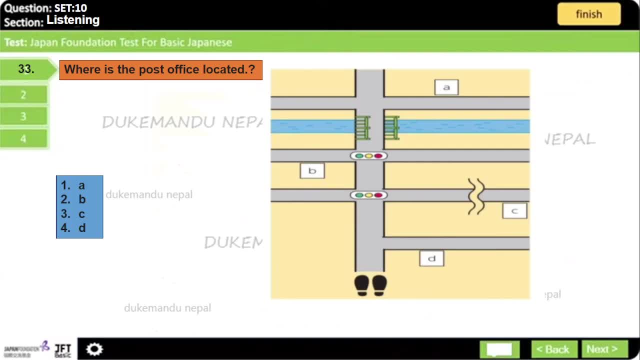 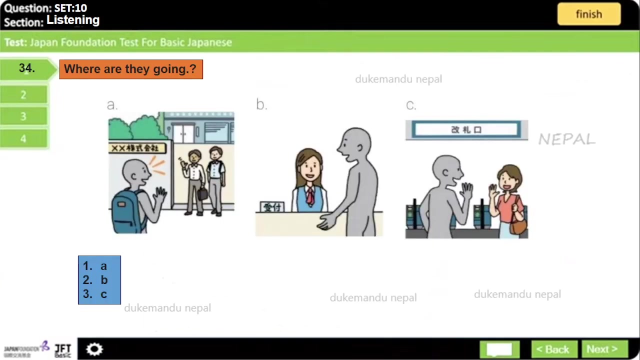 I'm sorry. What should I do to the post office? Go straight down this road and turn left at the second signal? I should go left at the first signal. No, it's not the first. 二つ目です分かりました. 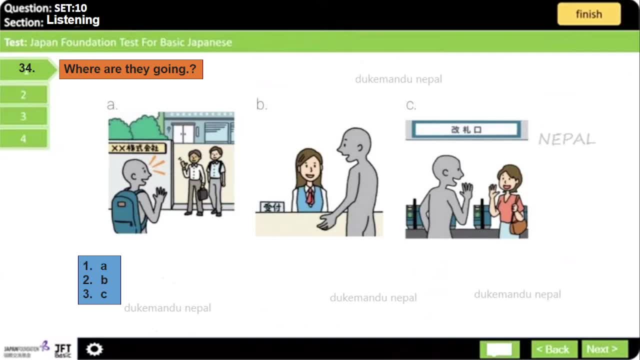 では金曜日の10時に来てください. 金曜日の10時ですね. えーと場所はどこですか? 受付に来てください, その後部屋に案内します. 分かりました. 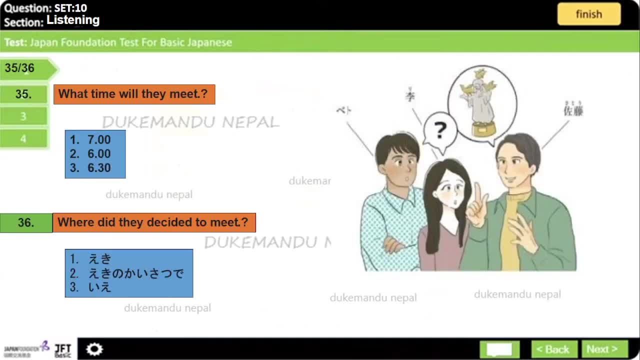 明日何時にしますか? 6時はどうですか? 6時はちょっと早いです, 6時半でもいいですか. 6時半いいですよ, じゃあそうしましょう. 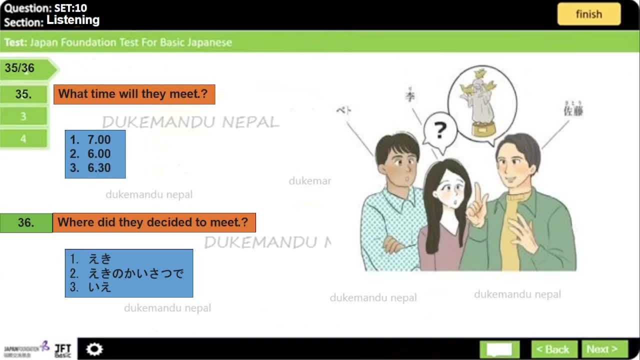 待ち合わせして一緒に行きますか. そうしましょう, どこにしますか? じゃあ駅前の平和の鳥の像の前にしましょう. 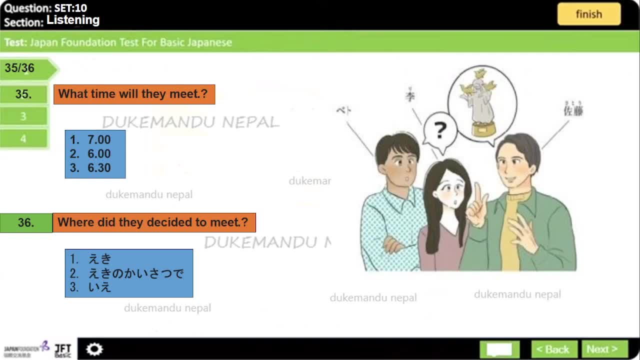 えそれ何ですか? 私も分かりません. 駅の改札でもいいですか, じゃあそうしましょう, 6時半に駅の改札集合で. はい, 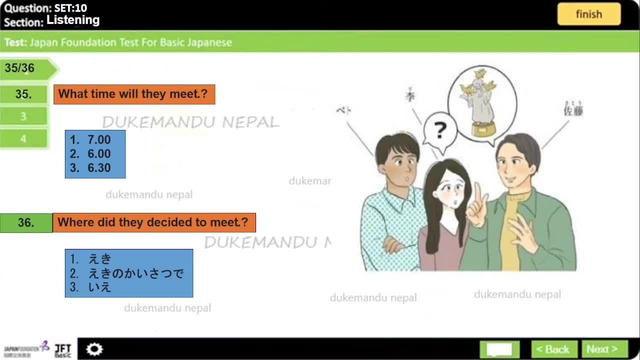 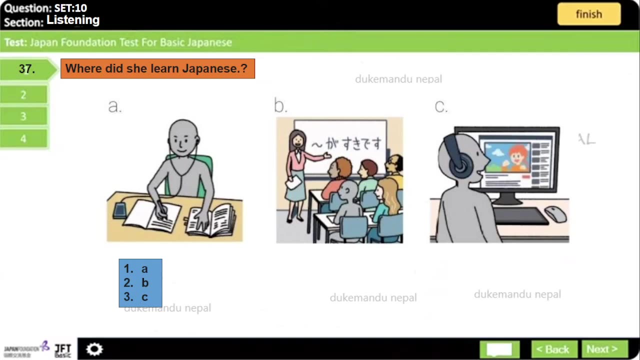 はい, 分かりました どこで日本語を勉強しましたか. 日本語学校で勉強しましたか? どれぐらい勉強しましたか? 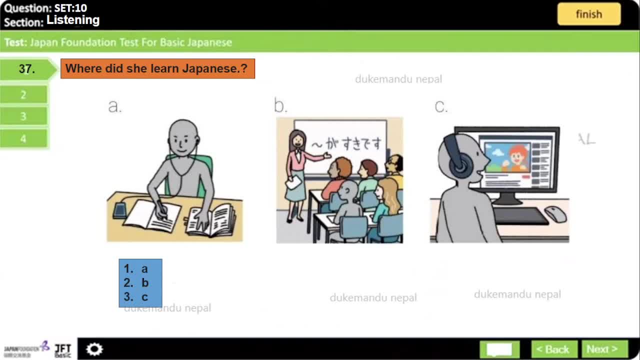 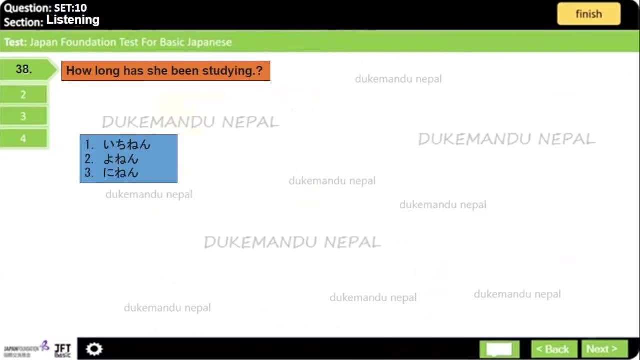 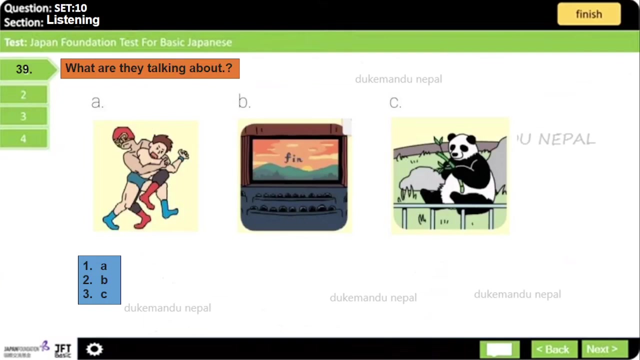 1年ぐらいです そうですか 日本語学校で勉強しましたか 1年ぐらいです- 動物園どうでしたか 楽しかったです. 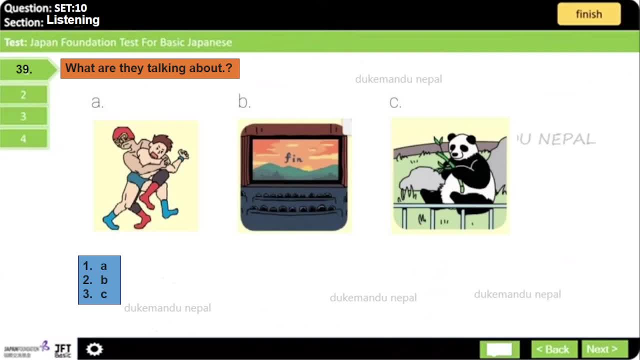 パンダが可愛かったです, 私は猿が良かったです. ああ猿も可愛かったですね. また行きたいです 駅前に駅前に出ました. 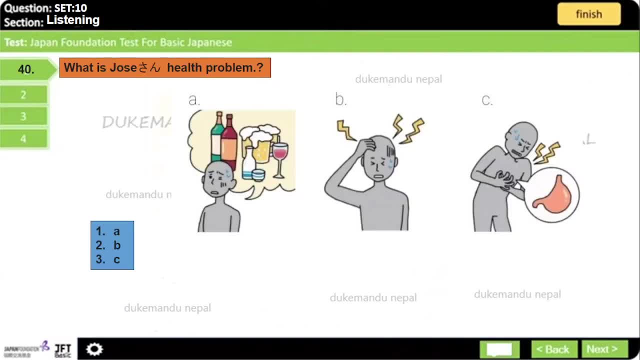 入り込んで駅を出始めて 駅を連絡したのですが 車が断られなくなりました. 駅前の車を通って行くだと. 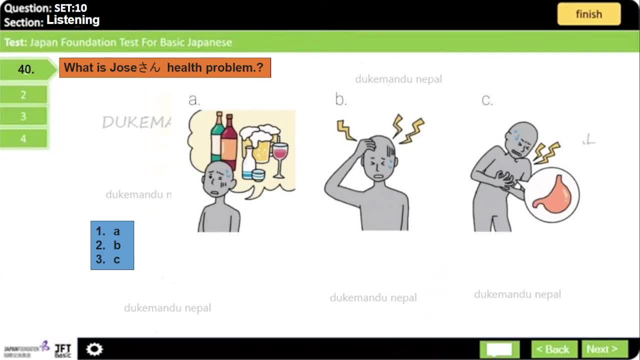 聞かれましたか. 先日は長い時間でお休みしました. お渡ししたいことはないのですが 昨日は飲み過ぎました. Sakai-san, what do you do on your second day of sleep? 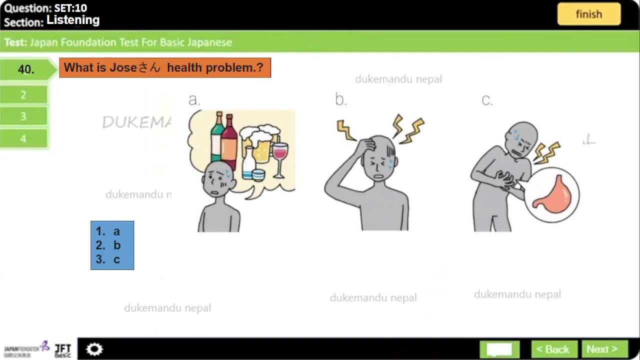 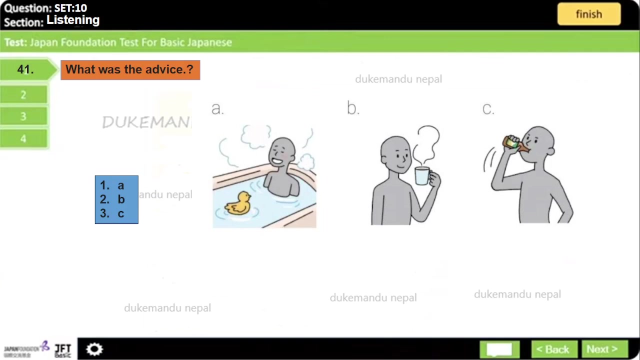 I drink medicine on my second day of sleep. It's pretty good, I see, But I like to sleep the most. That's right. What's the matter, Poopin-san? I haven't been able to sleep well lately and my body is tired. 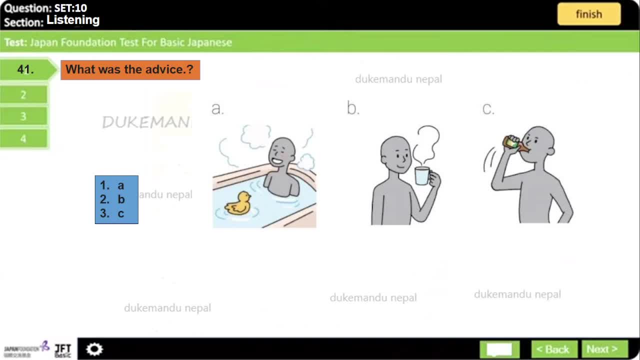 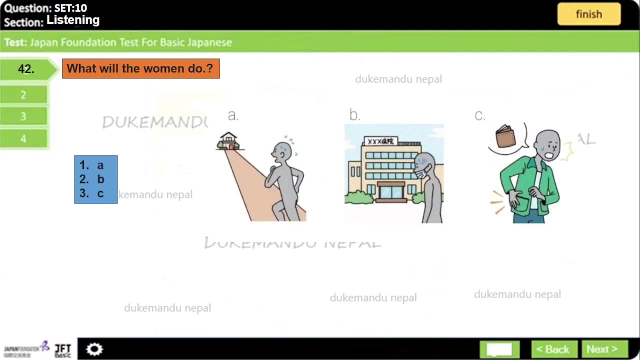 That's not good. When you can't sleep, well, it's good to take a warm bath, Is that? so I'll try it. Yes, this is Kitaburawa Hoos. Hello, this is Anissa. Yes, this is Anissa-san. 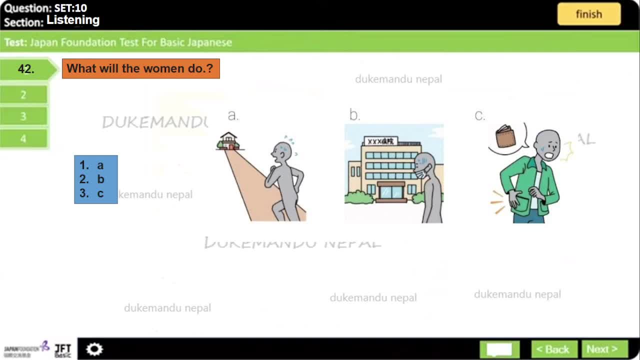 Excuse me. Yes, I left my wallet at home. I'm going back to pick it up now. I'll be back in a bit. Yes, I understand. Thank you, I'll take care of it. Thank you very much. 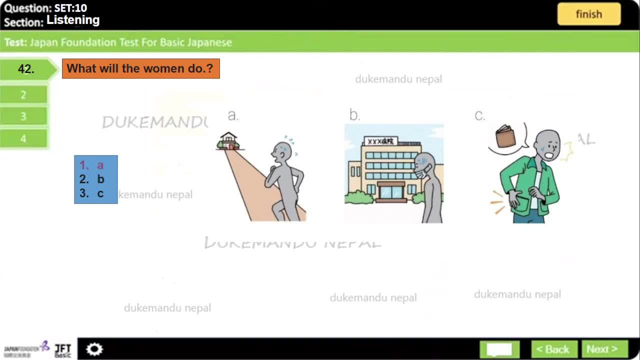 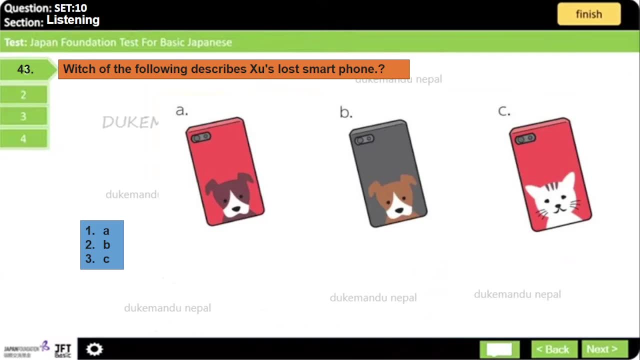 You're welcome. You won't be late. Alice'll take you there. Excuse me, I lost my phone. Did you get the reply? A smartphone. I'veまで your search done. Please tell me the features of the smartphone. 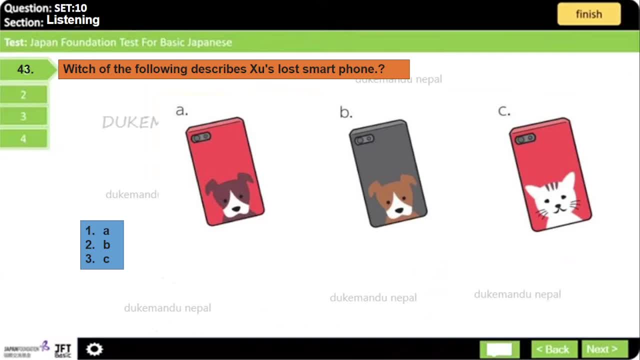 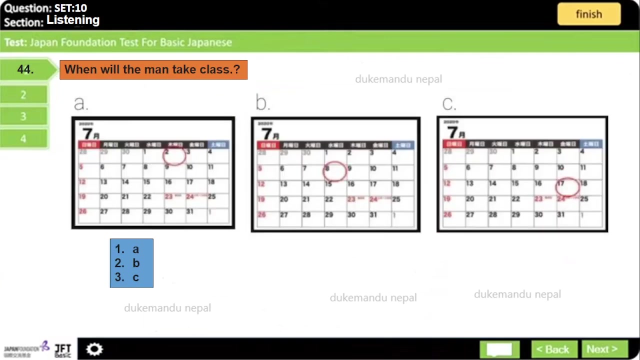 Well, the color of the smartphone is black and there is a red cover on the dog's face. I see What is the model: It's an iPhone. I'm sorry, I'd like to take part in this cooking class. Cooking class, I see. Please wait a moment. 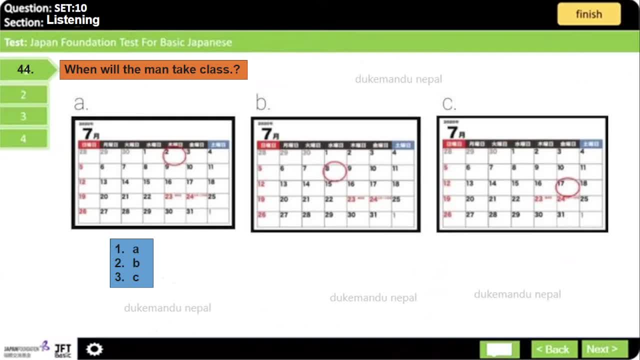 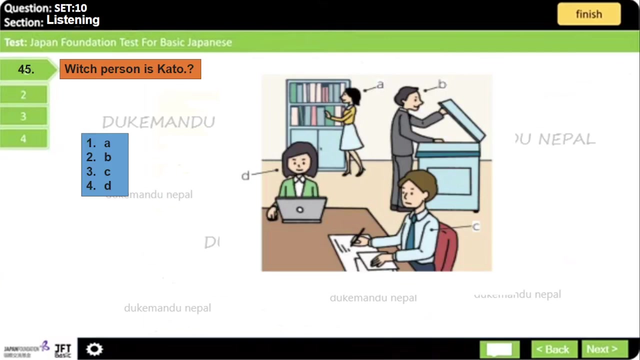 Oh, there are already a lot of classes on Friday. Can I take the Thursday class? Yes, that's fine. Um, how much is it? Please pay 800 yen once. Excuse me, is Mr Kato here? Mr Kato, Oh, he's over there. 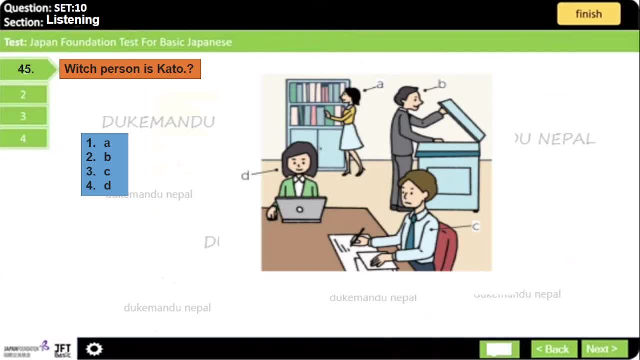 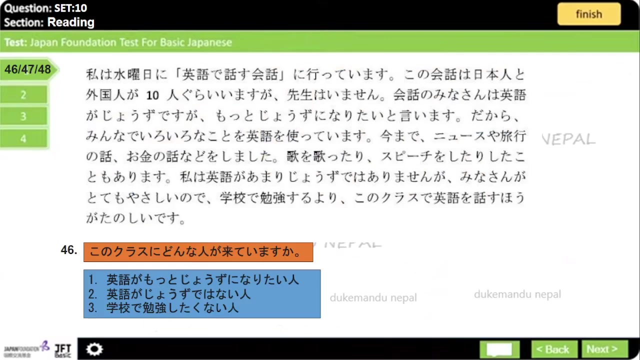 Eh, Who is he? Look, he's the one copying over there. Oh, I see, Thank you very much. She's very nice, You're welcome. Thank you very much. Thank you very much, You're welcome. Thank you very much. 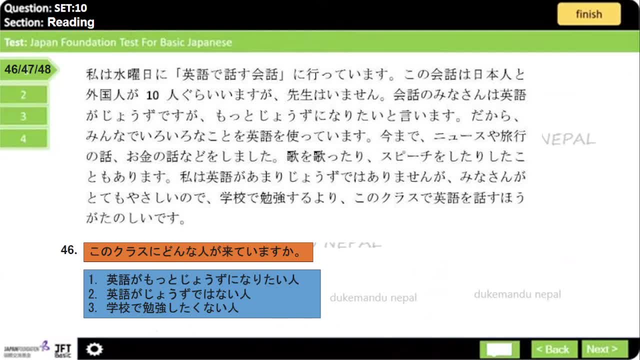 Thank you very much. Thank you very much, Ms Kato. do you have another question? What do you have to say to people who have no answer? Well, I like the way you talk. I'm sorry you Thanks for watching.